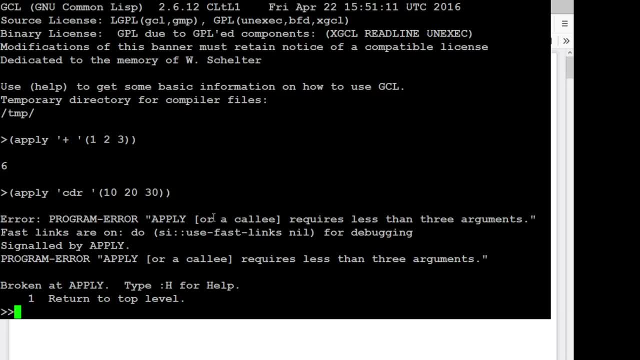 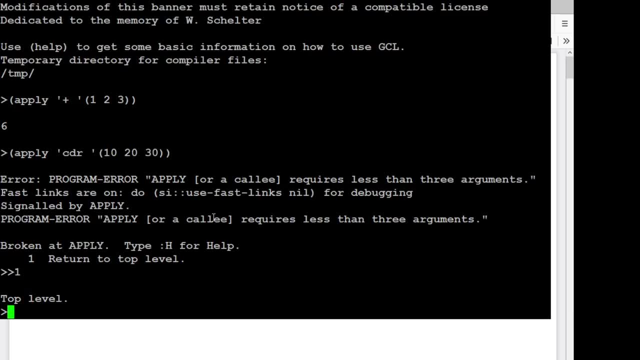 Oops, Oh, what have I provided here? Ah, okay, So cutter expects to get a list as its argument And apply expects to get a list that contains the argument. So I actually need a list inside a list here to do this correctly. 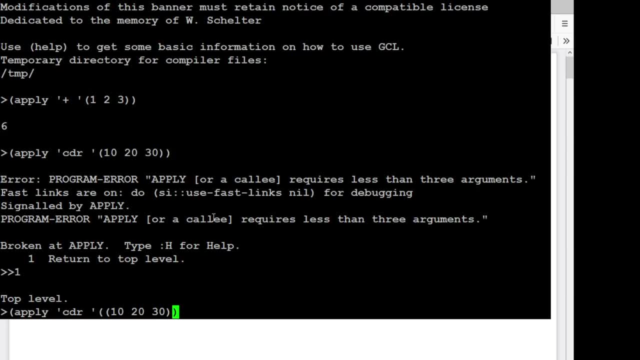 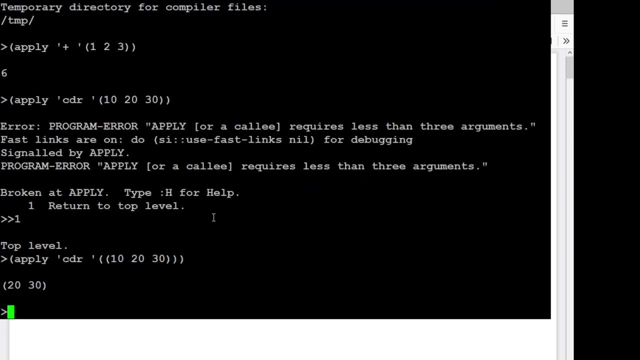 So I have to pass. So the arguments that are being applied or that cutter is being applied to is the list: 10, 20, 30. Ha, okay, there we go. That looks more like it, So we can go off and pass. 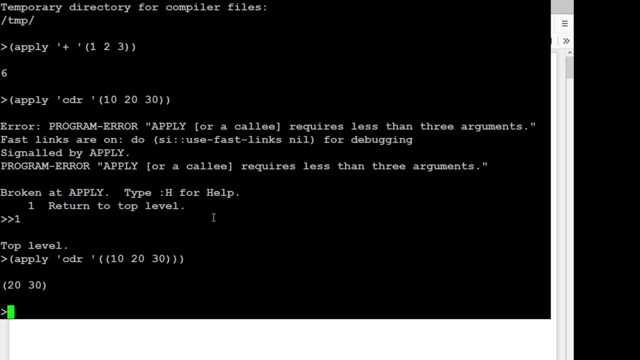 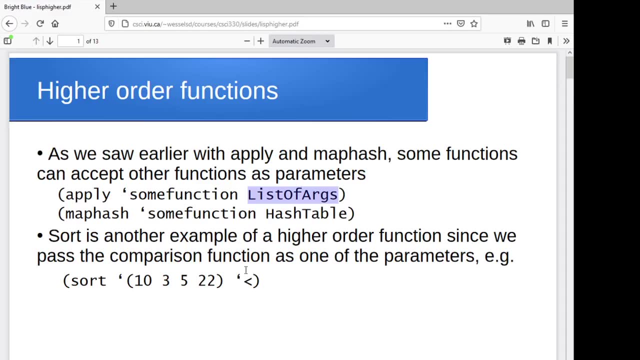 And then we can use the function as a parameter to apply and send it some data values to use or a list of data values to use, And it calls the function on those values All righty. Another example is the map hash function that we looked at earlier, where you give it some function. 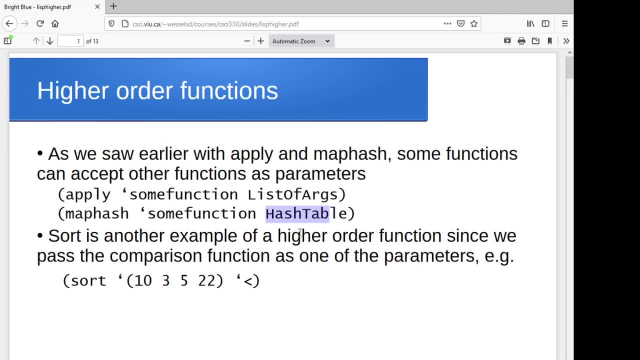 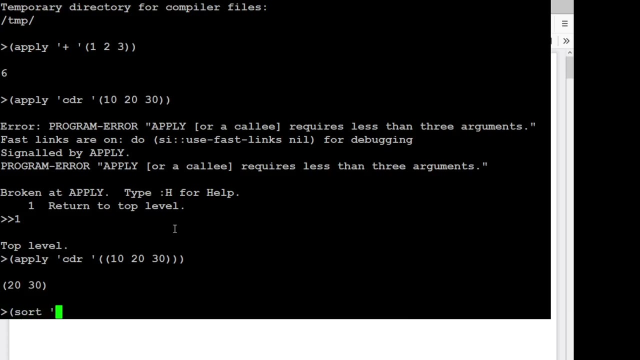 and it runs that function on every key value pair in the hash table. There's another one where we can specify: I want to sort some list of values and we specify what operator. So if we try a sort and I might actually need to specify what kind of data, I'm expecting the result as 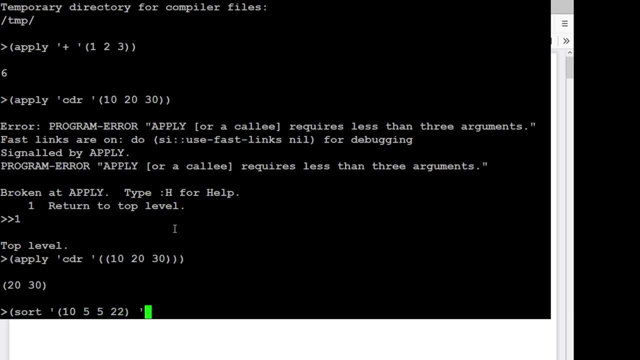 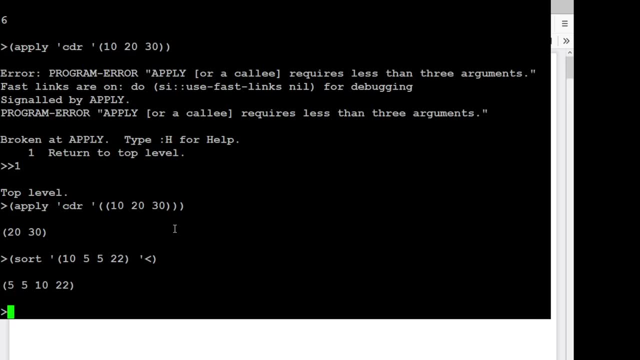 But let's give this a whirl: 5, 22.. So I'm saying, sort and use the less than as the comparison. So it goes through and sorts in ascending order And if I try that again using the greater than, it should sort in descending order. 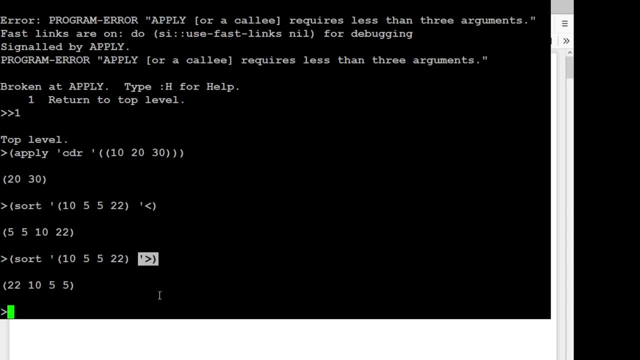 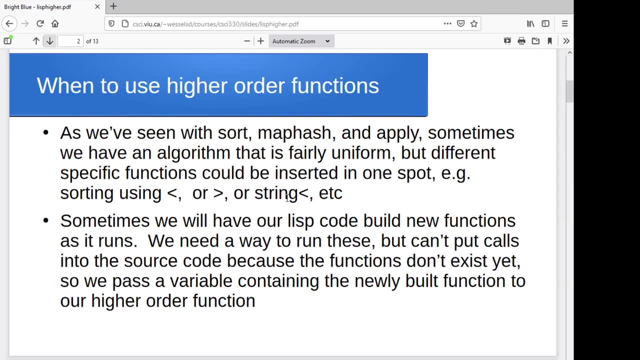 So again, I'm passing the function that I want to use for comparison as a parameter to my sort function. All right, So there's a variety of different places where we wind up using these. We're going to come up with some more creative uses of them very soon. 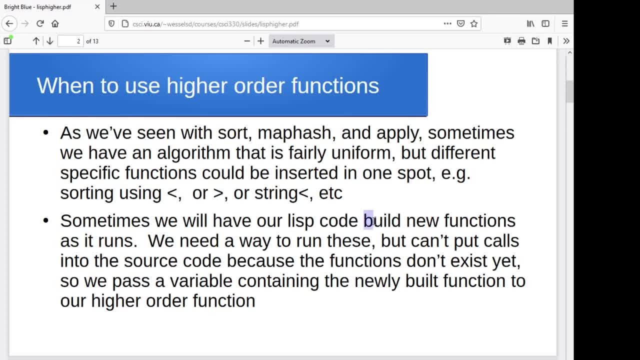 What we're going to look at are creating functions that build other functions and then, in turn, pass those off to be executed. So When we, when we do that, the new functions that we build in the Lisp code will be anonymous, sort of unnamed functions. 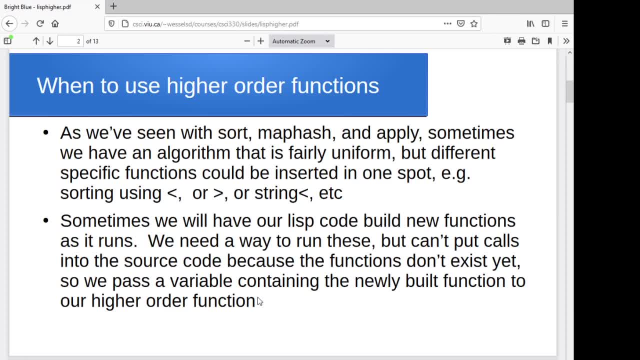 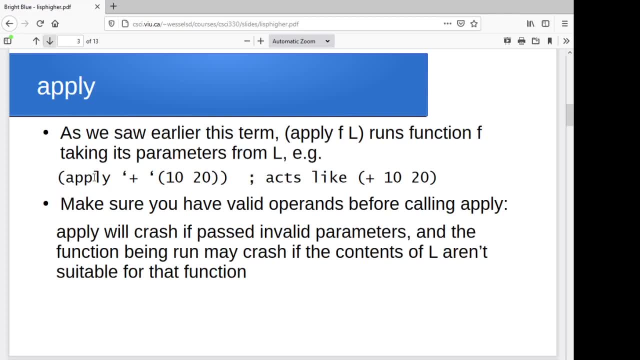 So we have to pass them as parameters to something else, since we can't call them by name in the source code. All right, So apply. we just ran through a couple of examples there where we say: apply, give it the function that we want to run, and we give it a list of data values. 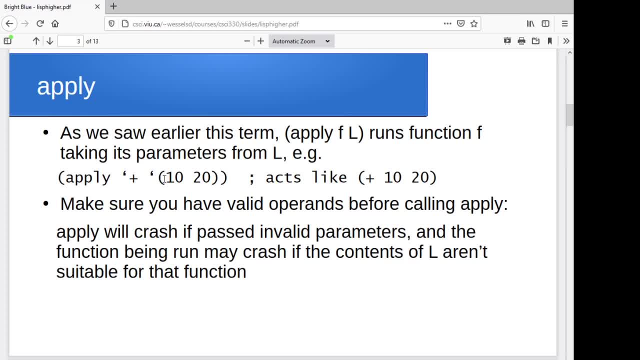 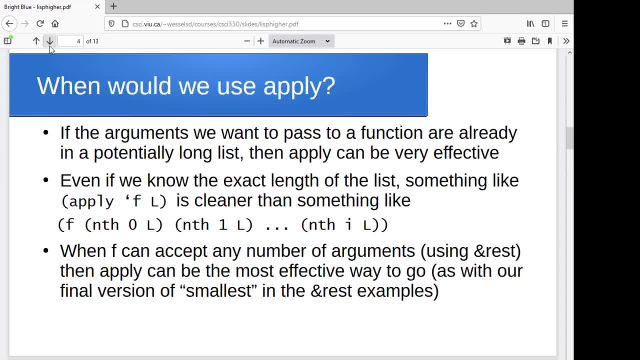 As the first element in running it as a function, right, And it's pretty much what's going on. So there are a variety of times when it can be cleaner to say, apply some function to a list. Um, we'll look at a variety of different circumstances fairly shortly. 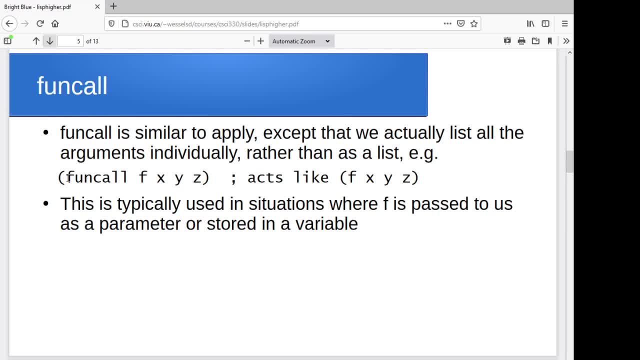 A couple of other variants that are useful. Fun call is very much like apply, except that instead of providing the arguments in a list, we just provide them directly in the function call. So, for instance, if we wanted to do, let's use our same example. 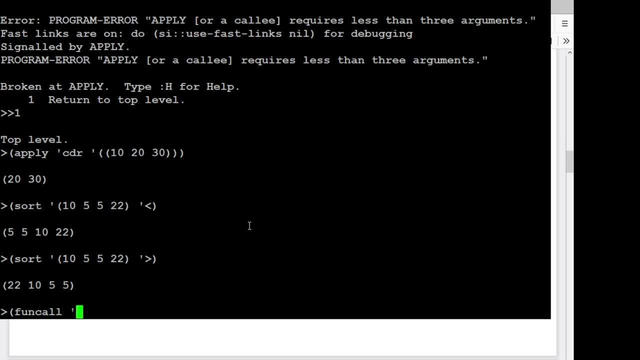 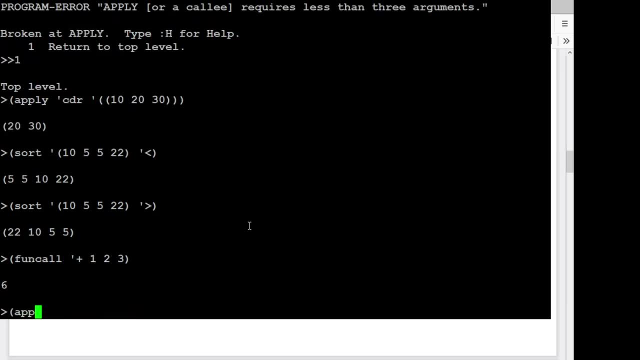 Let's say I wanted to do a fun call, but I wanted to do the sum of the values one, two and three. We just provide them directly, right, As opposed to apply where we said let's do it and provide the three of them in a list. 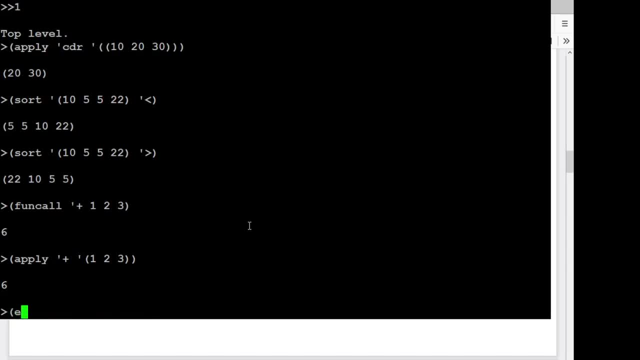 So very similar. Another variation that we're going to look at in one second here is eval. Another variation that we're going to look at in one second here is eval, where we give it the entire expression as a list and it goes off and runs it. 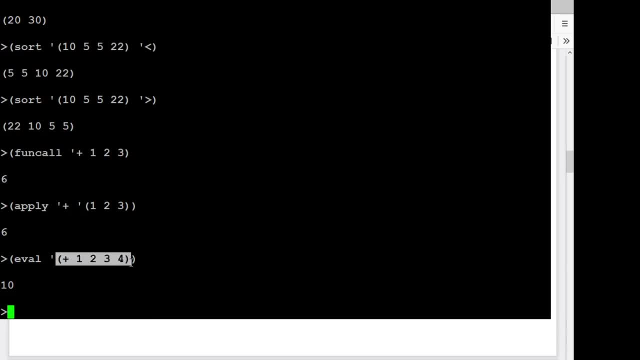 This is going to be useful in cases where we build the function that we want to run in Lisp, so we actually have code that builds that function and then we pass it off to eval to basically say, okay, well, what does this do? 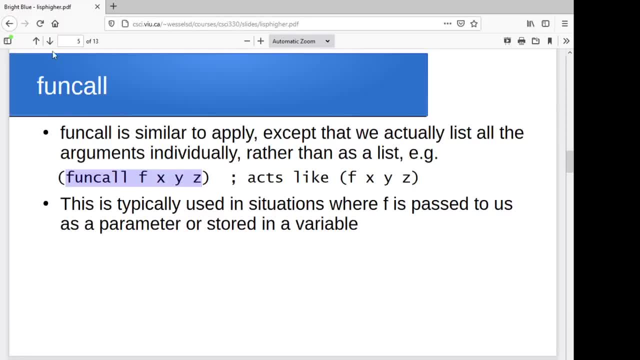 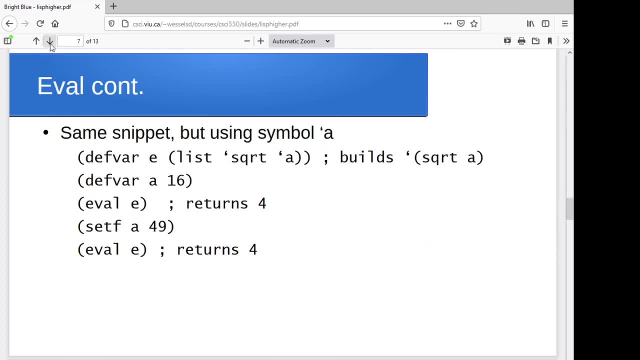 So this is the, or at least some of the ideas we're going to be playing with. So eval again, as we went through, it just goes through and evaluates the entire expression. So, assuming the expression is given to you as a list, 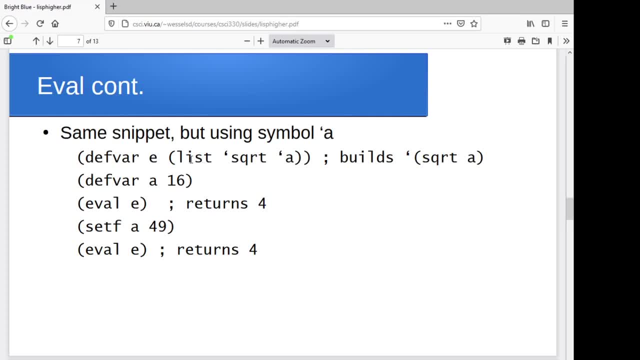 So just again, a variety of different ideas Here. we're going to create a variable that contains this list, that's got a symbol for a function and has a symbol for a variable, so it builds this list. square root of a. Then we'll go through and define a value for a and we'll evaluate e. 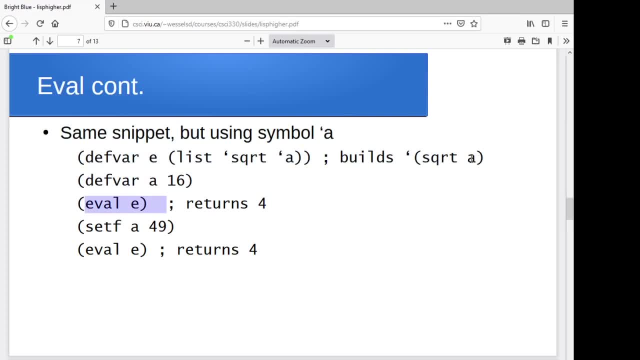 So we're going to go through and evaluate that expression. So it's going off and saying, okay, I'm going to go through and evaluate this expression. So it's going off and saying, okay, I'm going to go through and evaluate this expression. 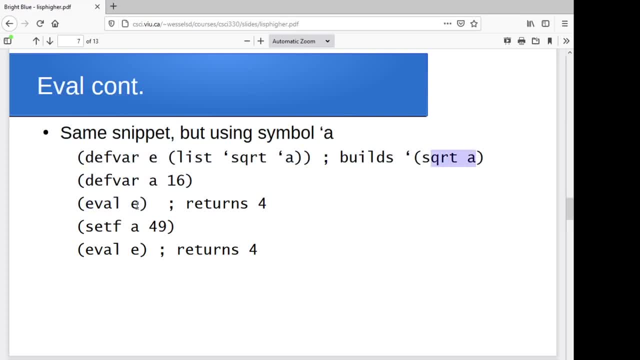 So I'm going to run this right. I'm going to evaluate square root of a, which, of course, by this point, since a now exists, is going to be 4.. Let's see, I don't think that last one is actually right. 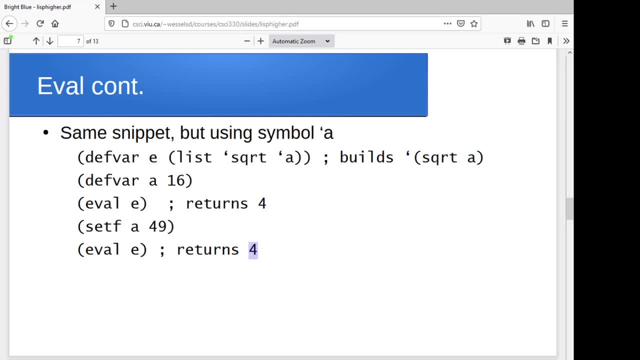 I think we should be returning 7, but let me just let's go through this. Def var e: the list of the square root Of a symbol, a. So if we look at what e is again, it's this list: square root a. 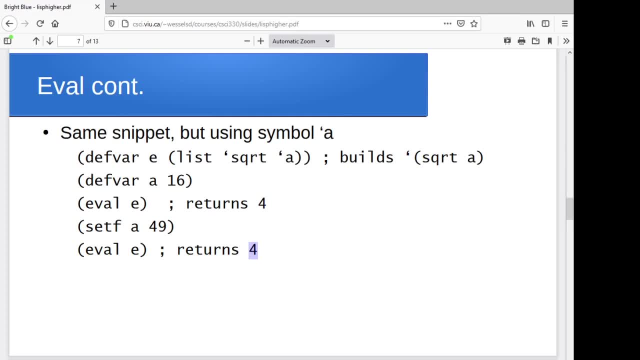 So if we go through and declare a and evaluate e, yay, And if we set f, a to 49, and we evaluate e, how about? we evaluate e, we get 7, right? So just to clarify, Confirm a typo in the slides there. 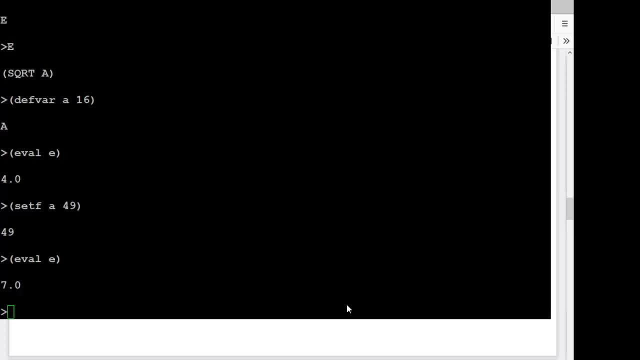 Oh, and I didn't show you any of that. Let's give that one more try. So this is what I just went through and did, just to confirm what was going on. We created our def var e. is this list exactly what we just went through on the slide? 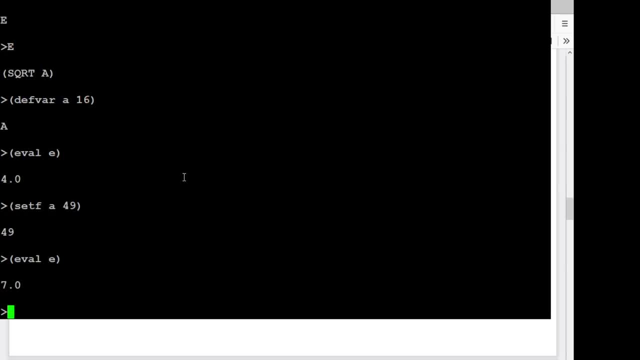 Just checked e to make sure that it was actually the square root. We went through and created our a, evaluated e, which is going to go through and do the square root of a and then changed. So we're going to go back to j and do our evaluation again and it changes the value of e to 7.. 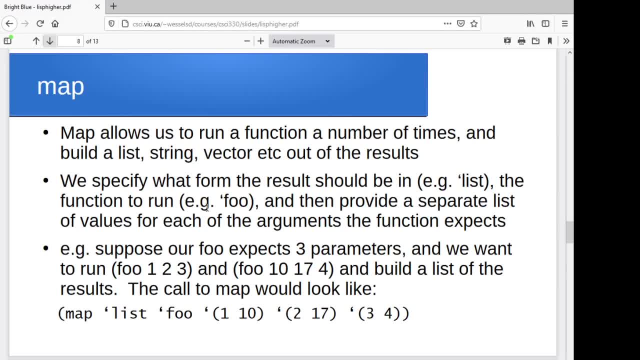 Alrighty. So a few more examples of higher-order functions. Map lets you run a function a number of times, but you're going to give it the parameters in lists. So what we'll do is, if we've gotten, let's say, a function that takes two parameters, 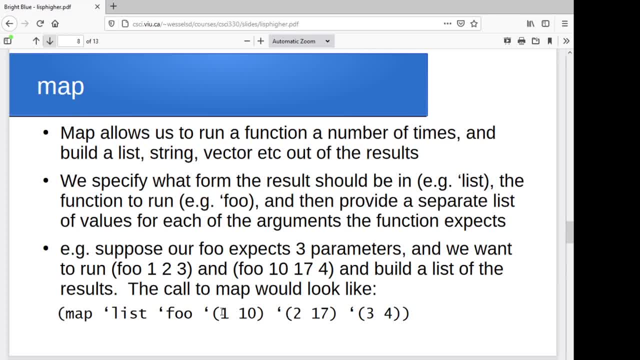 we'll give one list that has the first argument or a whole bunch of the first arguments. we'll give one list that has the first argument or a whole bunch of the first arguments and another list that's got the second arguments. So if I was, let's say, function foo takes two arguments. 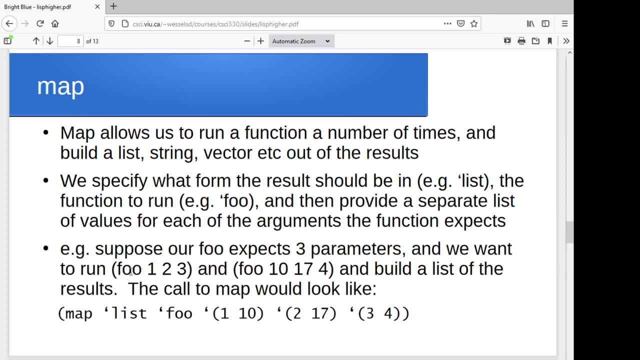 and or, pardon me, Here we've got a function- foo- that takes three. arg, Right, it's taking three arguments. I'll get myself right here. So we've got a function that takes three arguments. so what we're going to do is pass three lists to Map. 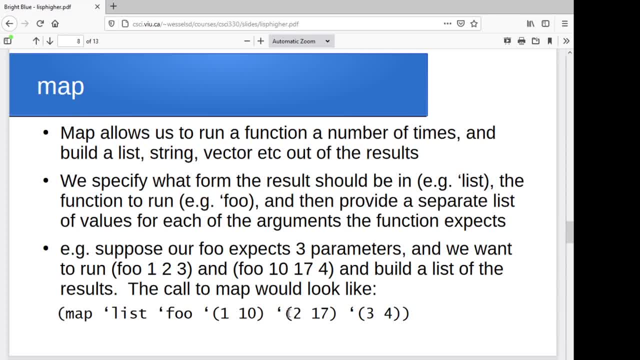 One That's going to be the values to use for the first argument, another list that's going to be the arguments to use for the values to use for the second argument, and a third list that's going to be the arguments to use for the third argument there. so what's? 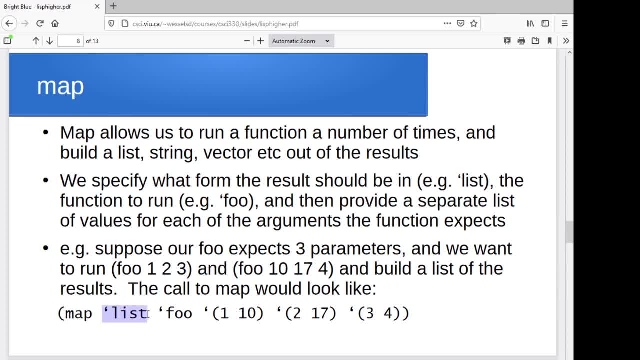 going to happen is when I run map, I'm going to say: please build a list out of the results. the function I want you to run is foo, and here are the data values. the first time I want you to run foo of one, two and three, and once you're done with that, I want you to run foo of 10, 17 and 4. 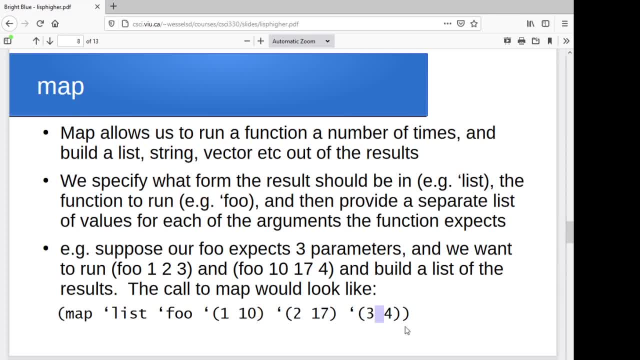 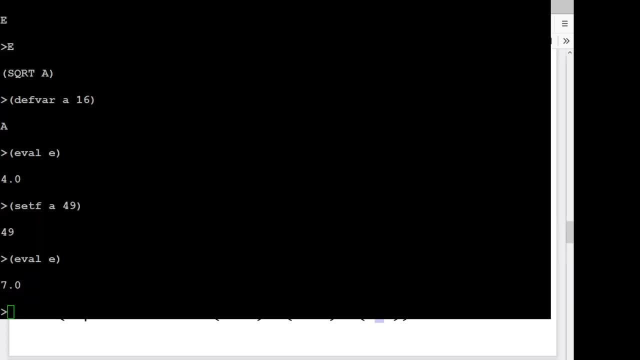 and we could have, you know, three values in each list, four values in each list, five values in each list, and it's just going to keep running foo over and over again, grabbing one element from each of the lists so slightly different again. so if we let's say, give that a try, let's try map. 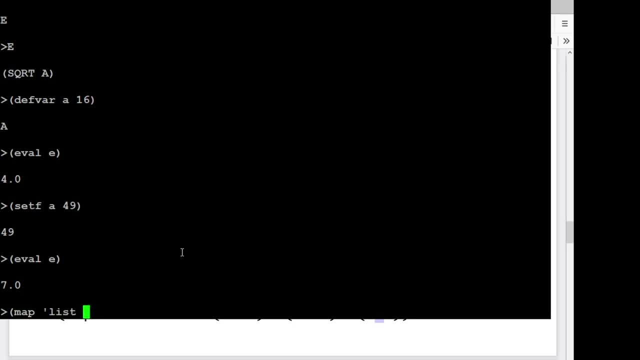 let's say, give that a try, let's try map. let's say, give that a try, let's try map, and we'll build a list out of the results. and how about? we'll make our function cons and so we'll give a list of the heads that we want to cons on to things. so let's say one, two, three, and we'll give a list of the lists that we want to cons things too. so let's say 10, 11 and 20, 21 and I don't know- 30, 31. 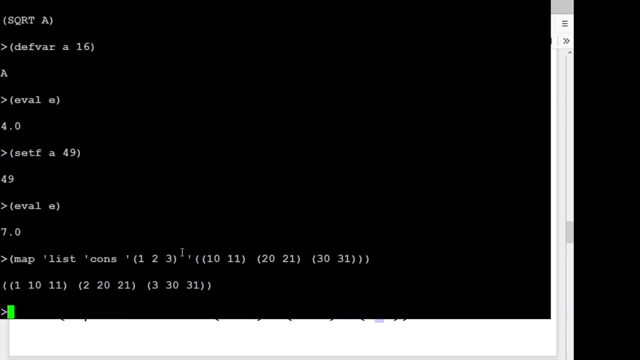 and it goes through and it takes that first one and cons it to the 10 and the 11, so it grabs that and then it cons is the 2 to the 20- 21 and it grabs that or creates that cons is 3 to the 30- 31. 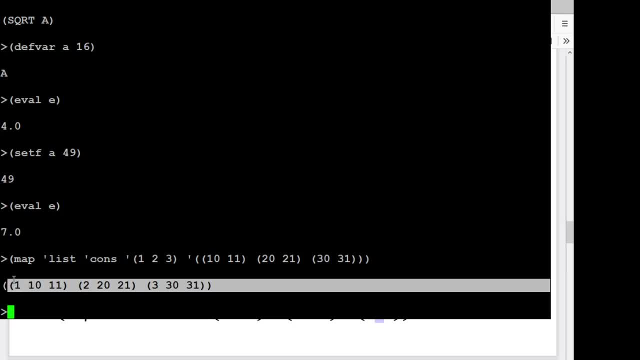 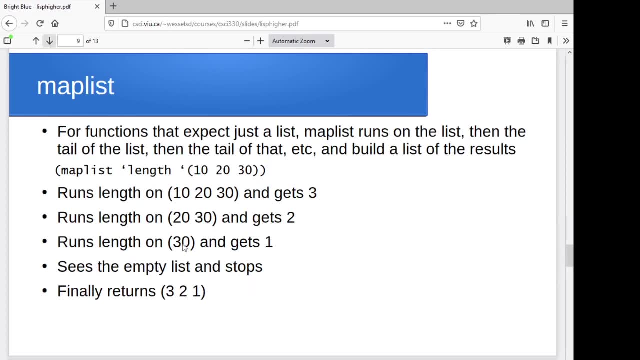 and creates that and then gloms them all together into a list. so map is another interesting one that we can play with. map- map of this is yet another interesting one. what does is runs a particular function on an entire list and then the tail of the list and then the tail of that list. 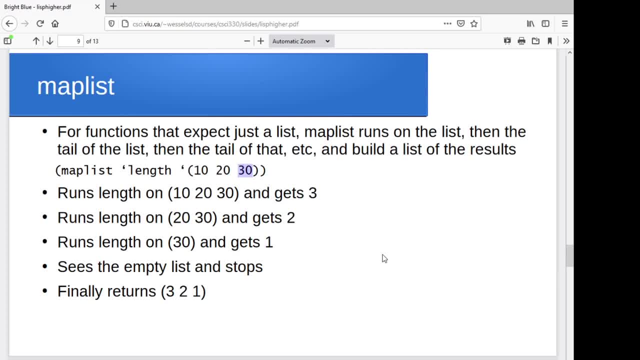 and basically just chopped off the head each time and running the defunction again. so for the link function we're showing here, we're going through and saying, OK, well, let's run it and grab the theuezner, the front element are pretty will run it and get a like the 3. we pull the ten-off in, room it again in. 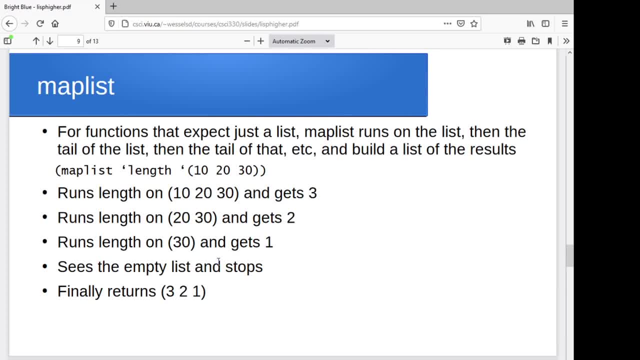 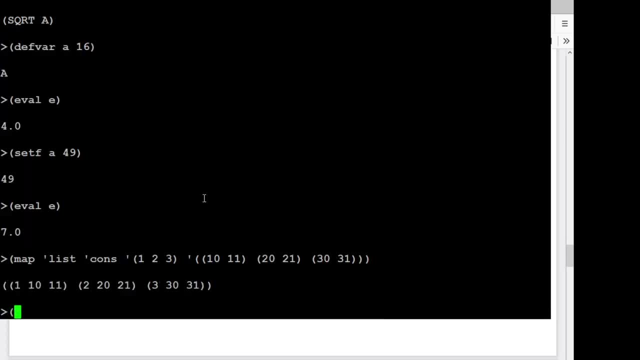 get-it- gepthed 20, we pull the next argument of run it again and get a length of one. So we want to go through and try map list on. let's try cutter this time. So we'll give it a list of just one, two, three, four, five or some such thing. So it 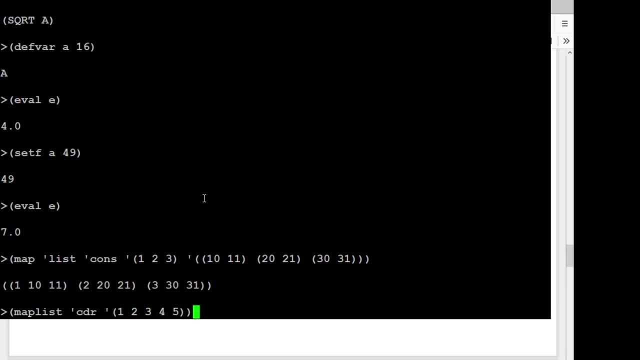 should go through and give me. the first thing it should give me is the list of everything minus the one, And then it pulls off the one and gives me the list of everything else, And we just keep going on smaller and smaller lists. right? The first time we call it, we get two, three, four, five. 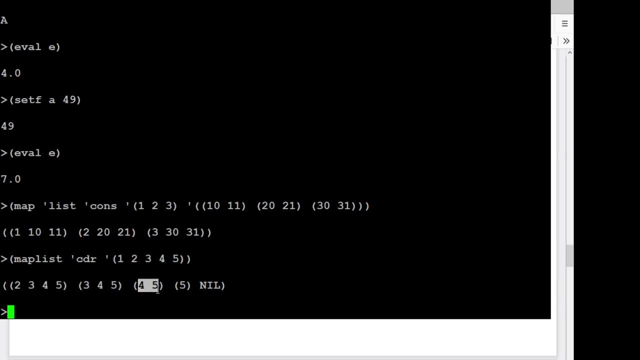 And then, with the one gone, we get three, four, five. And then, with the two gone, we get the four, five, With the four gone, we get the five, et cetera, et cetera, et cetera. Last call is just. 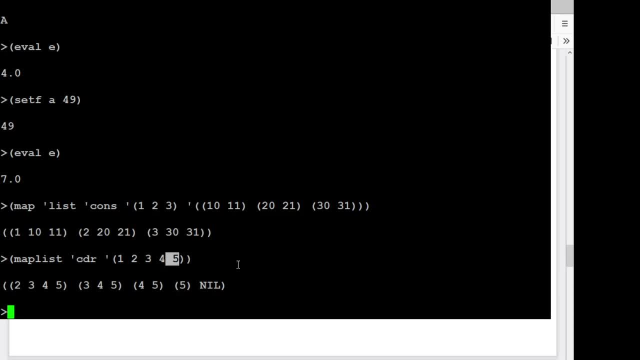 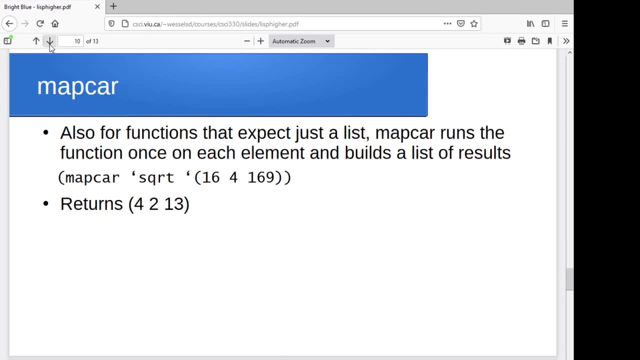 that one element list. So there are a ton of different higher order functions that Lisp provides And, depending on what we're trying to accomplish, we'll pick one or another of them. Map car is just another one, Another one that you provide a function and a list and it runs that function on each element. 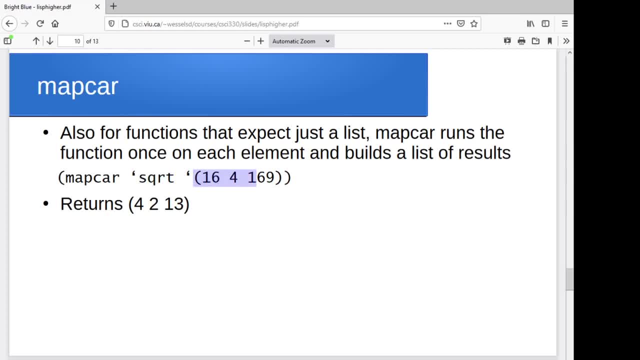 and creates a list of the results. So if I was to go through and say map car, and let's just use the minus and let's take our handy dandy, one Oops, Ah, one Oops. I'm not showing you this. 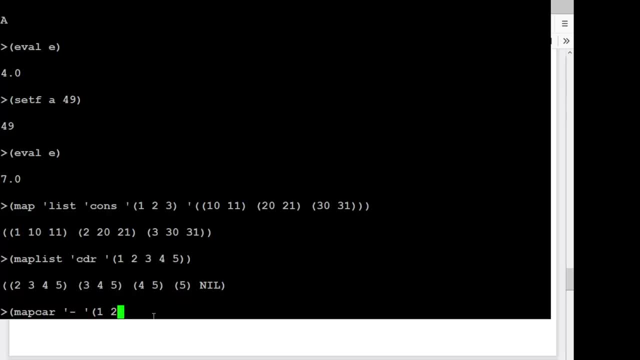 am I. So we'll try map car and we're going to use the minus operation, the negate operation, and we'll get the result. So we'll try map car and we're going to use the minus operation and we'll give it a list of one, two, three, four, five, And it should just go through. 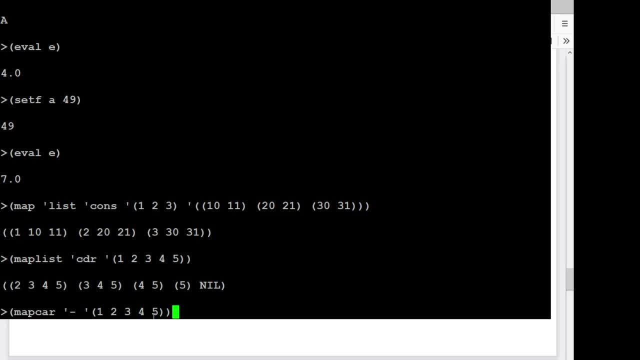 apply the negative to each element in there and give me a list of the results, right? So we get negative one, negative two, et cetera, et cetera, et cetera. So again, all sorts of different higher.